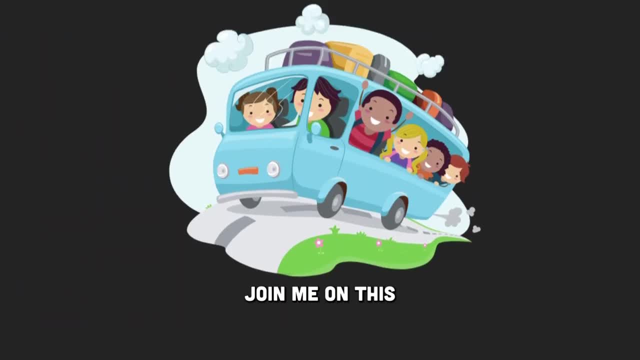 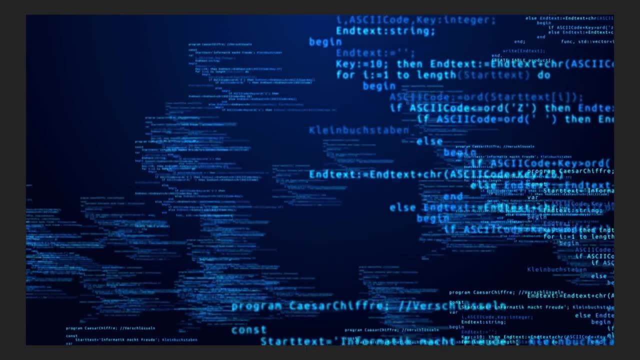 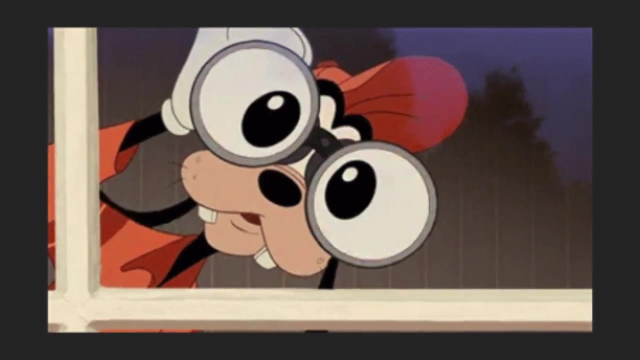 unwritten decree that held immense power. Join me on this thrilling journey as we unravel the mysteries behind this unspoken rule. In the enchanted realm of software engineering, ethical considerations play a pivotal role. But what exactly do these ethics entail? Let's embark on a quest to discover the three fundamental principles that guide software. 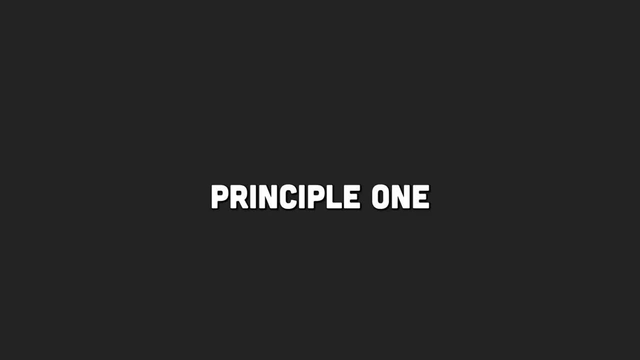 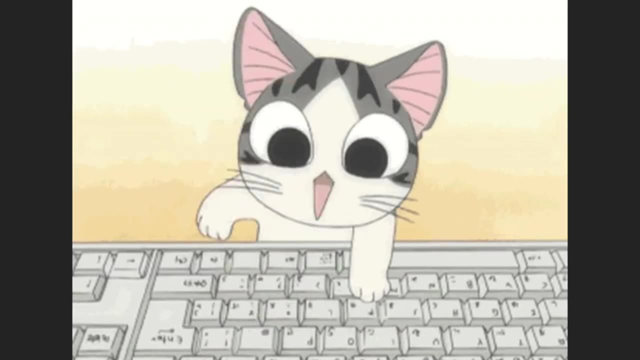 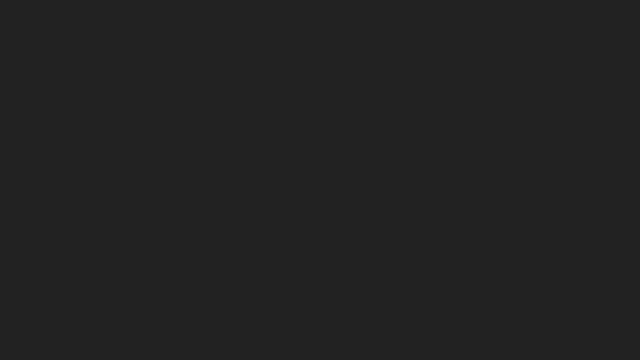 engineers in their virtuous endeavors. Principle 1. The Code of the Users. Our first principle is a noble one: a code dedicated to the users. Software engineers wield their keyboards with the intention of creating remarkable experiences, safeguarding user privacy and preserving the sanctity of their data. They understand that. 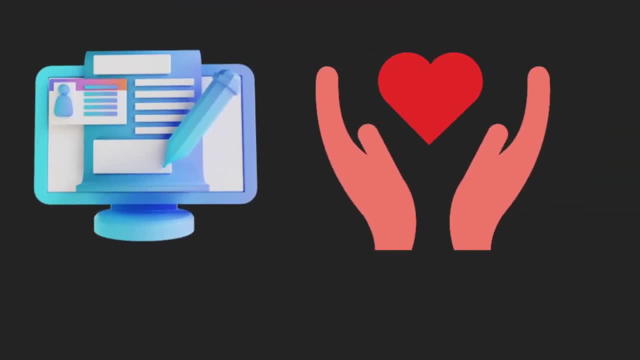 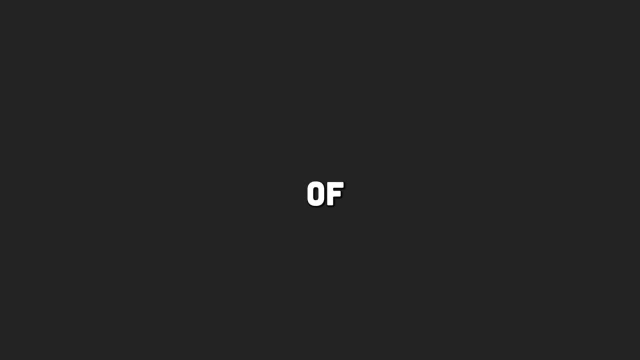 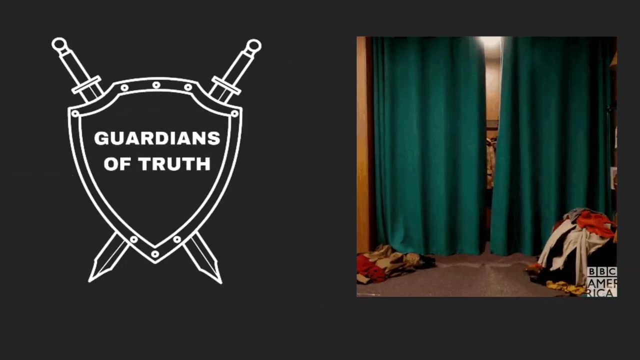 their creations hold the power to shape lives and prioritize the happiness and satisfaction of their users above all else. Principle 2. The Guardians of Transparency. Our next principle introduces the concept of transparency and accountability. Software engineers become guardians of truth, unveiling the intricacies of their code for all. 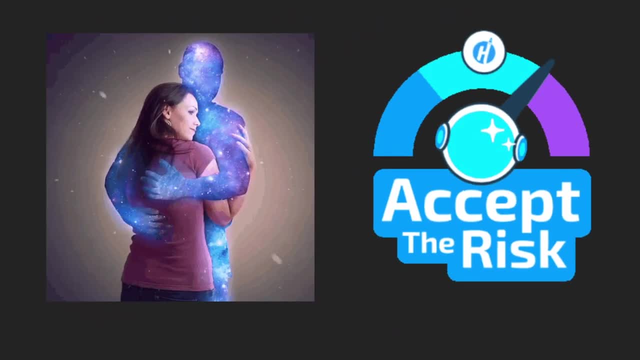 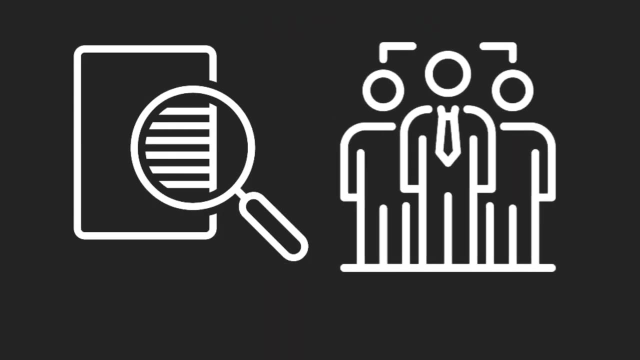 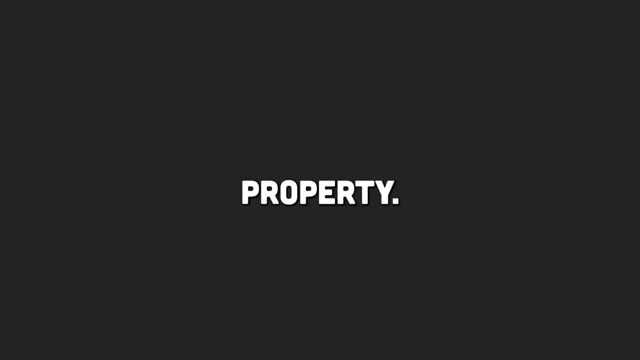 to see They embrace the responsibility of highlighting potential risks and limitations, ensuring that their digital creations serve as beacons of honesty. With transparency comes accountability, as they stand ready to face any unintended consequences that may arise. Principle 3. The Knights of Intellectual Property. The final principle introduces us to the noble 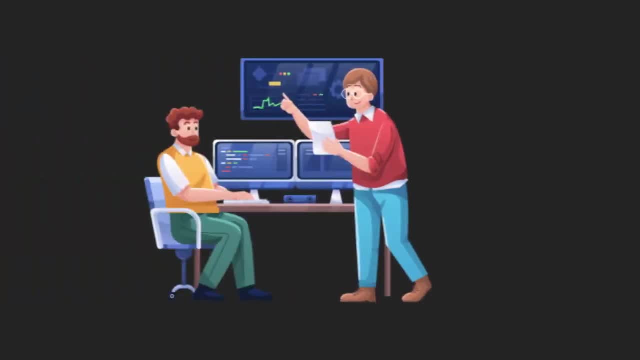 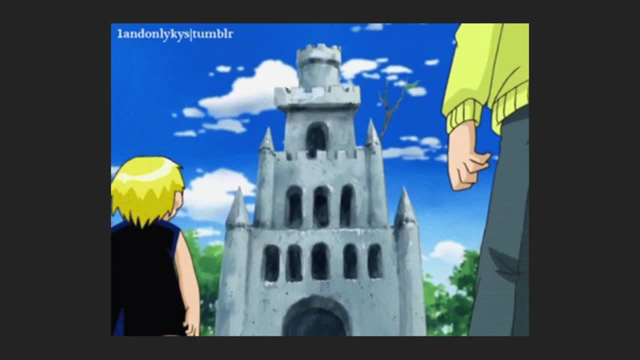 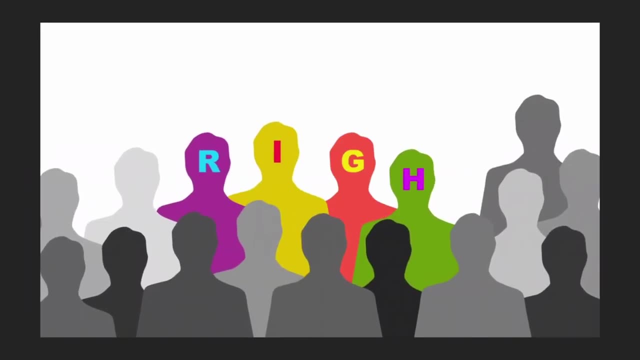 Principle 5. The Knights of Intelligence, They areoon to the ruptures of the rails of the human race. by respecting copyrights, patents and licenses, They build a fortress of respect and understanding, fostering an environment where innovation flourishes without compromising the 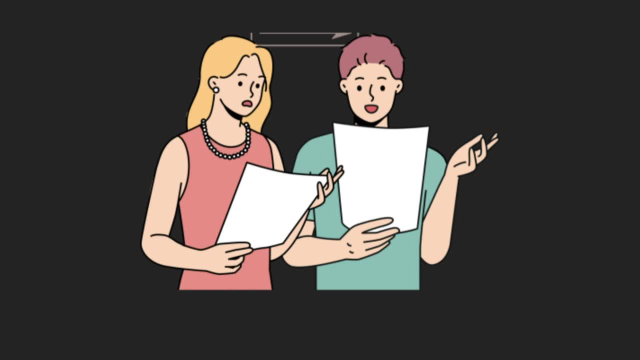 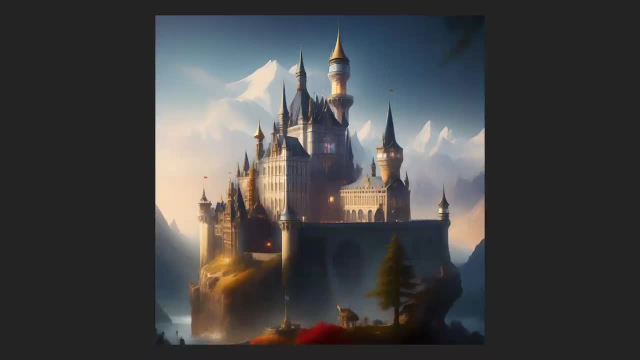 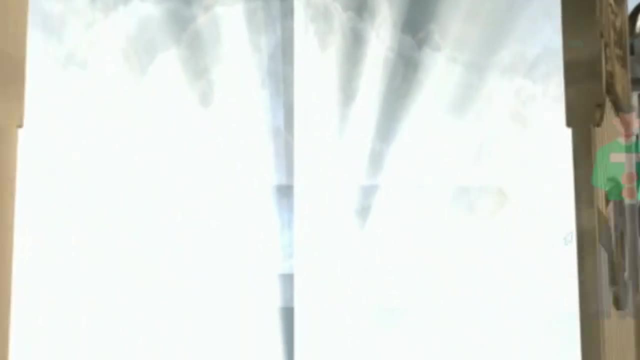 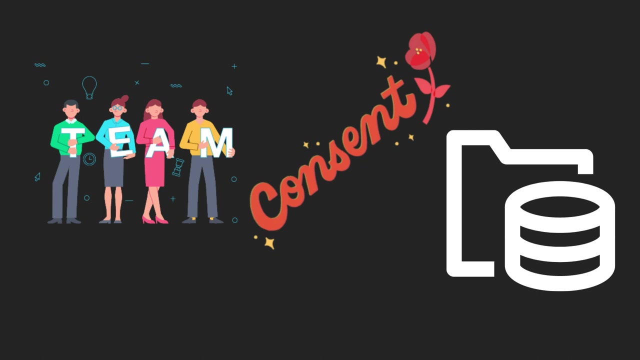 rights of creators. THE PENETRATING många mechanical cereales and intelligent debates. 맞아 areoonan al-seder Hazeacious If you are country manu. When the Tassel gates open, we witness a development team hard at work, ensuring that the explicit consent of users is obtained, their data encrypted and stored securely. 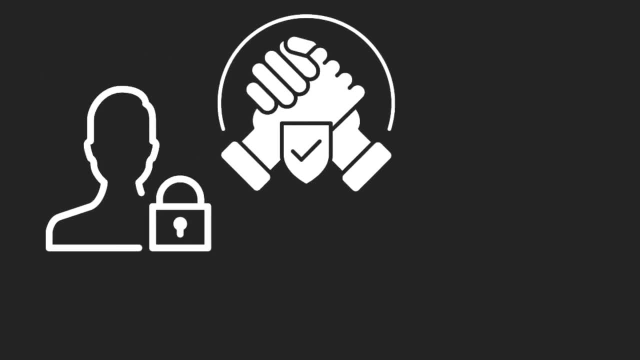 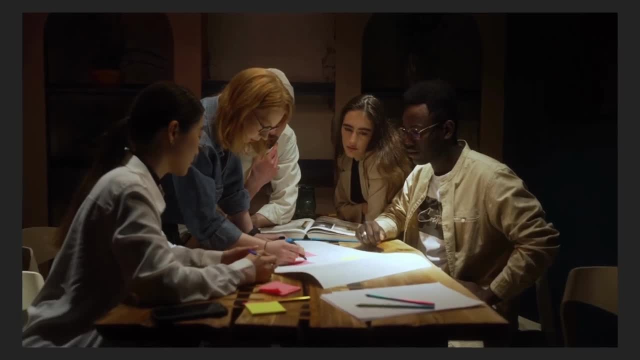 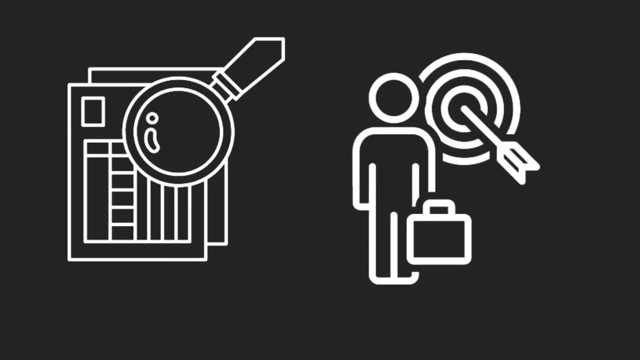 The company's commitment to user privacy shines as a beacon of trust, setting an example for others to follow The quest for fairness In a distant realm. a team embarks on a perilous quest to develop an AI-powered recommendation system. They tread carefully, testing their algorithms rigorously and employing diverse datasets to avoid falling into the clutches of bias.